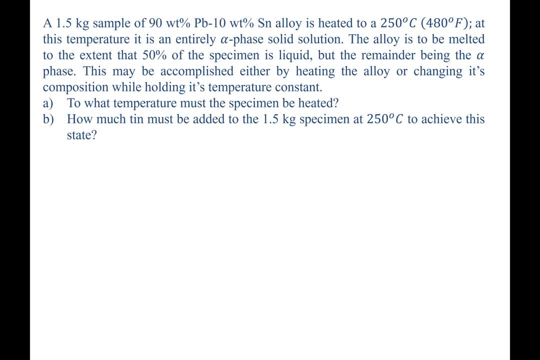 For this problem. we are told what the initial mass of a sample is: 1.5 kg. We know what the initial composition is: 90 weight percent lead and 10 weight percent tin. And we know that it's been heated to 250 degrees C, which places it in a single phase region, a region which is entirely alpha phase. solid solution, mixture of those two elements. 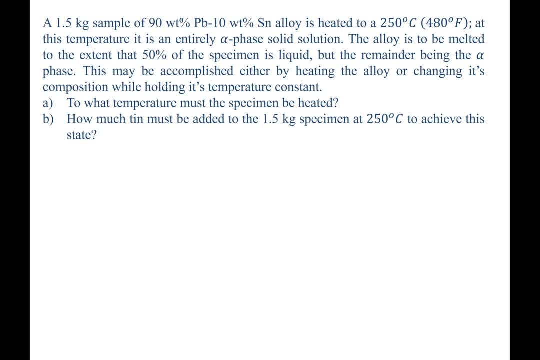 The question then goes on to say, if we wanted to melt this alloy such that it's 50% liquid and 50% solid, that that can be done in one of two ways. It can either be heated, keeping the composition constant, or we can keep the temperature constant and change the composition. 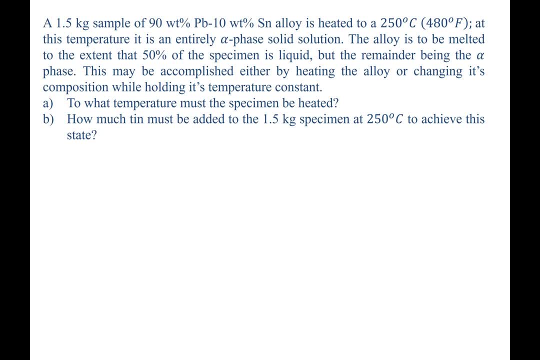 So part A asks: to what temperature must the specimen be heated? Part B asks if, instead of heating it, we wanted to keep the temperature constant. how much tin should we add to achieve the same result? So let's take a look at our phase diagram. 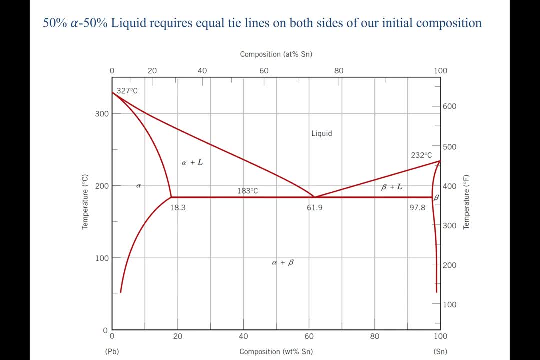 The phase diagram for lead and tin. Tin is shown as follows. It's a binary eutectic. Now let's find out where we initially were. We said initially that we had 10 weight percent tin and 90 weight percent lead at 250 degrees C, which places us right here. 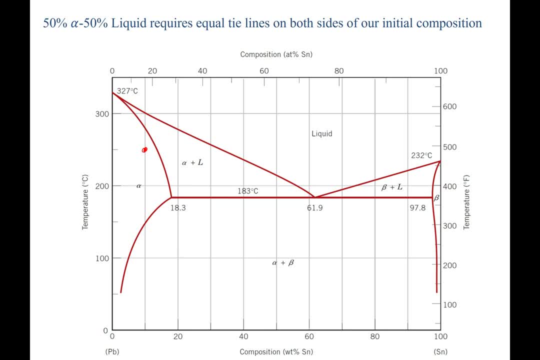 So for part A, we're just going to heat the sample up. We're going to stay along this gray line, So let's draw a line along there. And we want to identify the temperature at which the sample is heated, So we're going to draw a line along there. 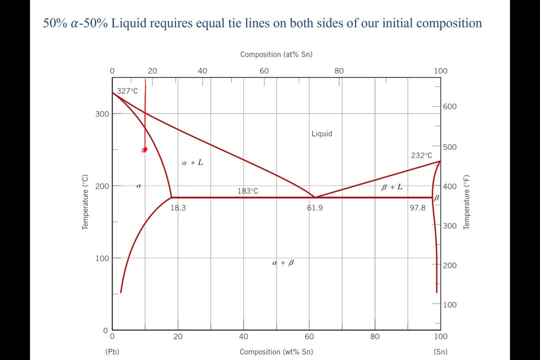 And we want to identify the temperature at which the sample is heated, Which, if we drew tie lines to the left and right, they would be more or less equal, Perhaps right there, Which is somewhere around maybe 290 degrees Celsius. So that would be the answer to part A. 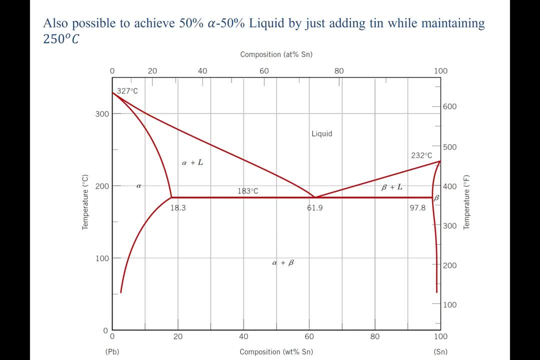 For part B, though, we know that we can just add tin to achieve the same result. So the first step is going to be draw a horizontal line at 250 degrees Celsius and identify where it intersects. the solidus and liquidus lines will allow us to determine the composition of the solid and the liquid form to that temperature. 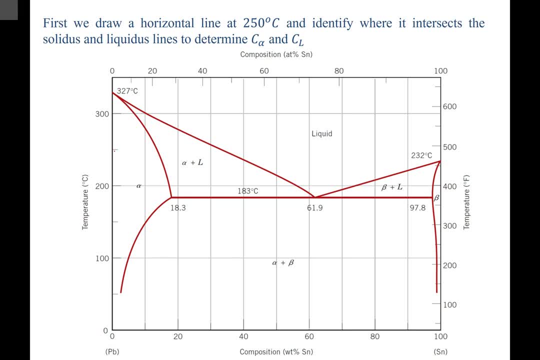 So drawing a horizontal line from 250 degrees C, like so, and then we drop, tie lines down to identify their compositions And looking at where those intersect the x-axis. it looks like the composition of our solid is, the solid form is going to be around maybe 14 weight percent tin, whereas the composition 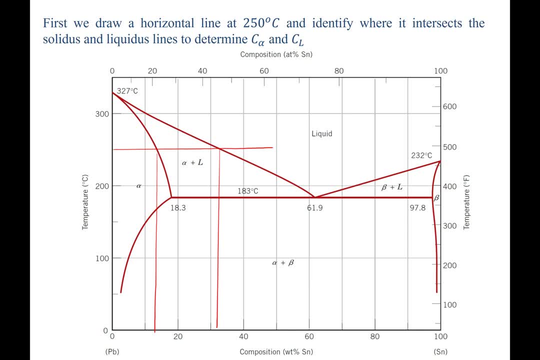 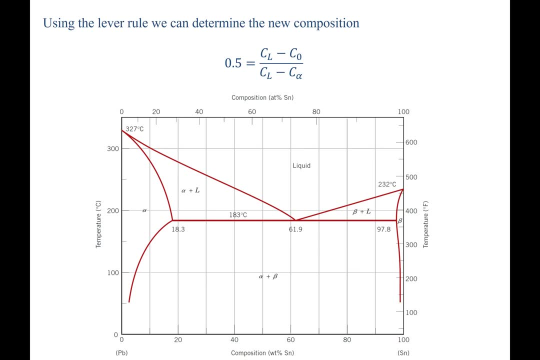 of our liquid that's formed is maybe around 33 weight percent tin. Now that we know those values, we can use the lever rule to determine our new composition, the composition at which we're going to have 50% solid and 50% liquid. 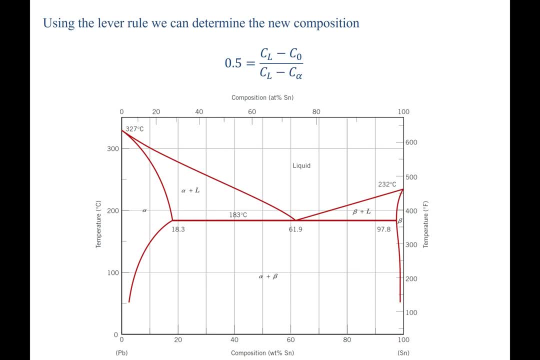 So 0.5, since we want 50%- will equal the composition. So we have the composition of the liquid minus the initial composition. Remember, graphically this looks like this: We have the liquid composition, we have the solid composition. We know our composition that we're looking for is going to be somewhere in the middle. 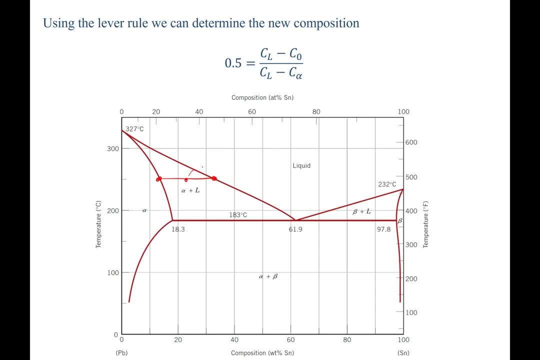 there. So we're figuring out this length of that line, that's C? L minus C naught, And then it's going to be divided by C L minus C alpha, which is the length of this total line like so. So, plugging in the values that we determined. 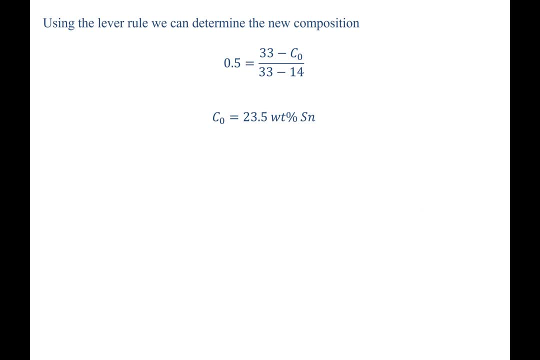 Previously. we have 0.5 equals 33 minus C naught and this is divided by 33 minus 14.. Solving for C naught, we find that it's 23.5 weight percent tin. So we know what the new composition needs to be, but the question doesn't ask for the 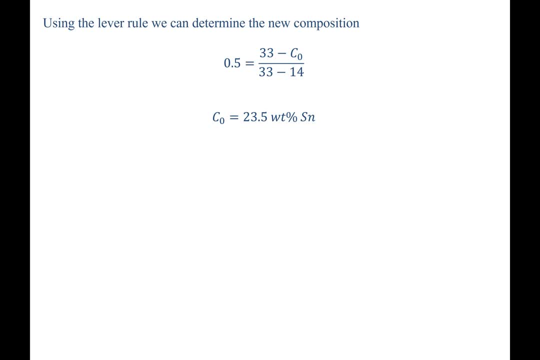 composition. It says how much more tin needs to be added to achieve that. So let's figure out how much tin we initially had in our sample, In our original sample, the amount of tin present, since it was a 10 weight percent tin and we had 1.5 kilograms. 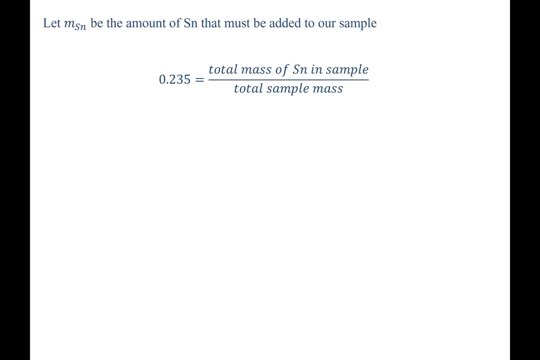 We had 0.15 kilograms- Okay, 0.15 kilograms of tin initially. Therefore, let's let M sub S N be the amount of tin that has to be added to our sample To achieve a composition of 23.5 percent or a fraction of 0.235, that would be equal.